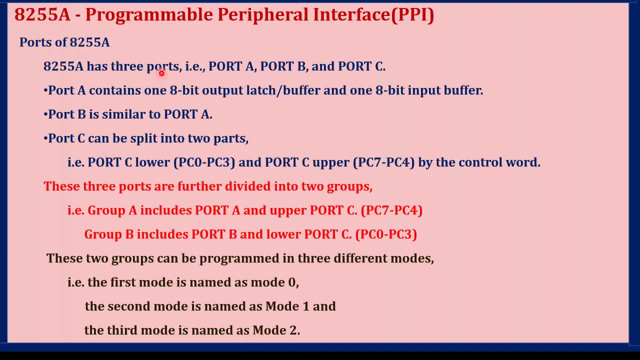 Let us see ports of A255A. Each port is having 8 lines. Those are port C. Those lines can be used to transfer the data from input device or transfer the data to the output device. So port A contains two buffers. One buffer is used as an input buffer, Another buffer is used as an output buffer. 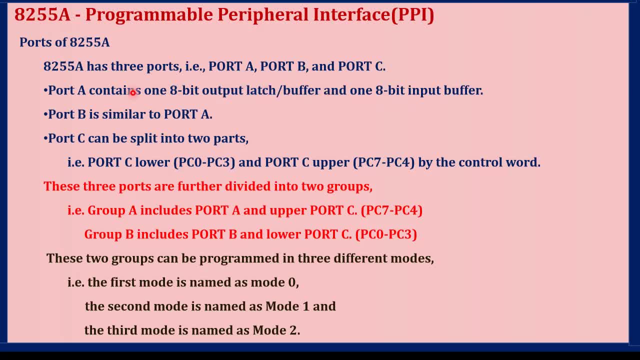 The size of the buffer is 8 bits. Similarly, port B, Port C, Port C. So in case of port C, the lower bits and upper bits of the port C can be split. Okay, we can use this- port C lower bits and port C upper bits separately. 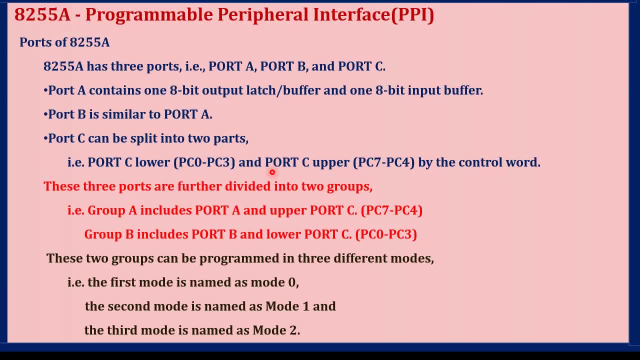 Means we can transfer 4-bit data also. So these ports again divide. Divide it into two groups. I told you group A, group B. Group A consists port A and upper port lines of port C. Group B contains port B and lower lines of port C. 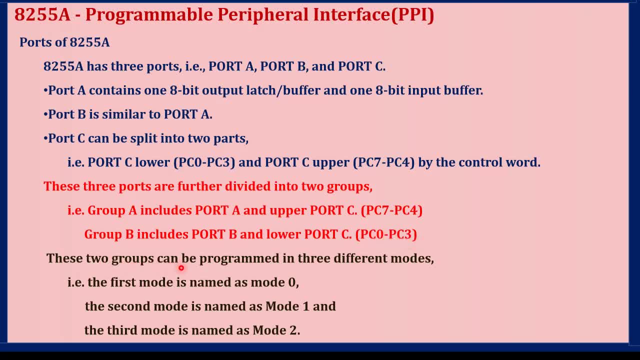 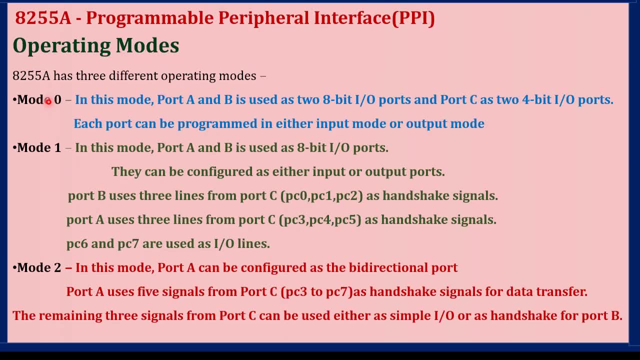 That is PC0 to PC3. These two groups can be programmed in three different modes. Those are mode 0, mode 1, mode 2.. We can say 8255.. We can operate in three modes. In mode 0, port A, port B, port C are used as input or output ports, according to our requirement. 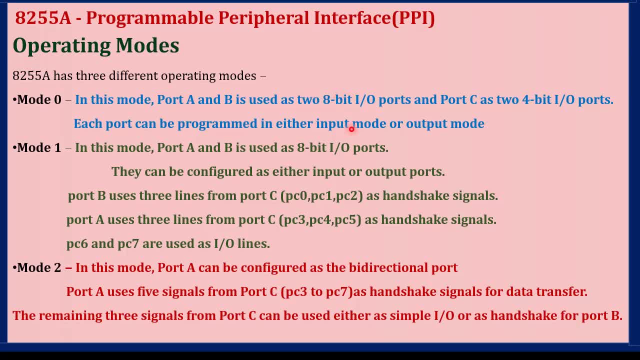 We have to program those ports in either in input mode or output mode. In mode 1, port A, port B are used as I-O ports. They can be configured as Either input or output ports. In this case, port B uses three lines of port C as handshake signals. 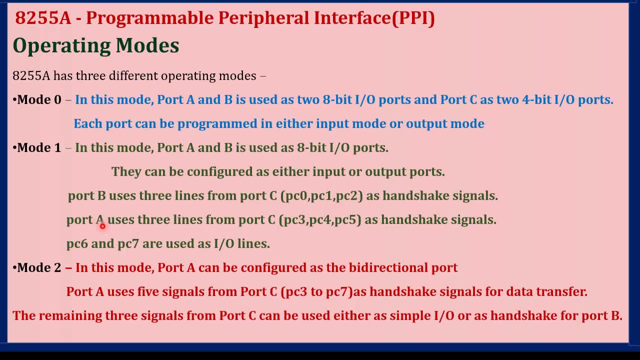 Those are PC0, PC1, PC2.. Port A used another three lines of port C as handshake signals. Those are PC3, PC4, PC5.. Okay, here PC0 to PC5 lines are combined. They are covered. remaining PC6, PC7 are used as normal I-O lines. 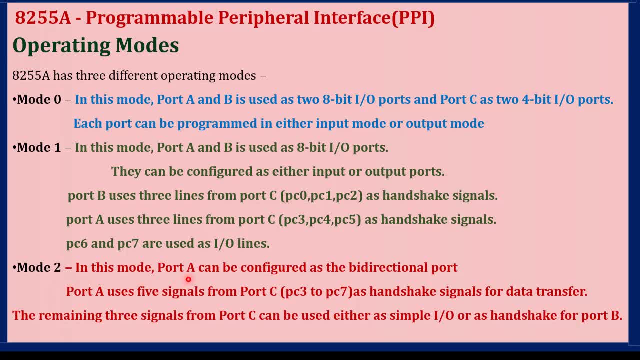 Okay, in case of mode 2, port A can be used as bidirectional port. Bidirectional means it can receive the data. It can send the data through those lines. Port A uses five lines of port C as handshake signals for transferring the data. 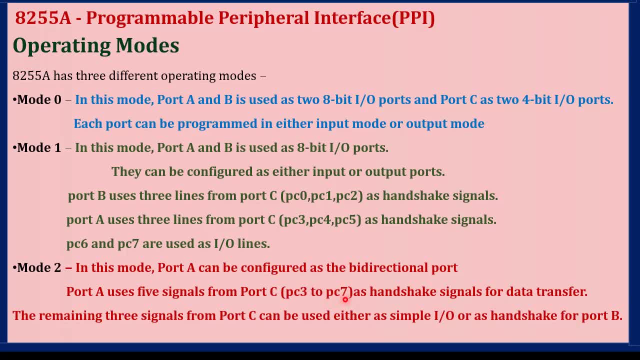 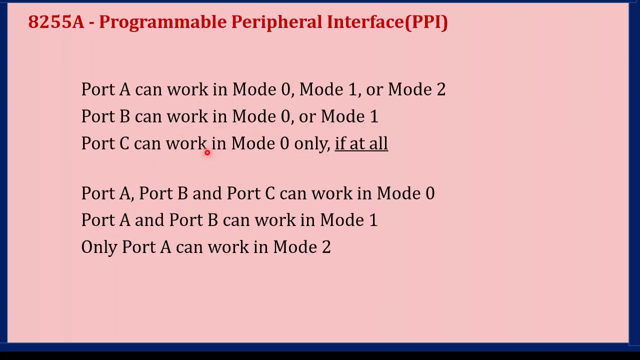 Those are PC3 to PC7. Five lines. The remaining lines of port C can be used either as I-O lines or handshake signals for port B. Okay, so you have to remember all these modes. Ports are operated in different modes. Okay, if you summarize the operation of ports in different modes. 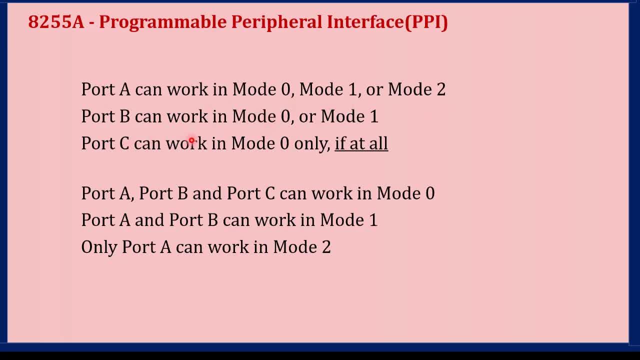 Port A is used in mode 0, mode 1, mode 2.. Port B is used in mode 0 and mode 1.. Port C is used in mode 0.. In mode 0, port A, port B, port C are used. 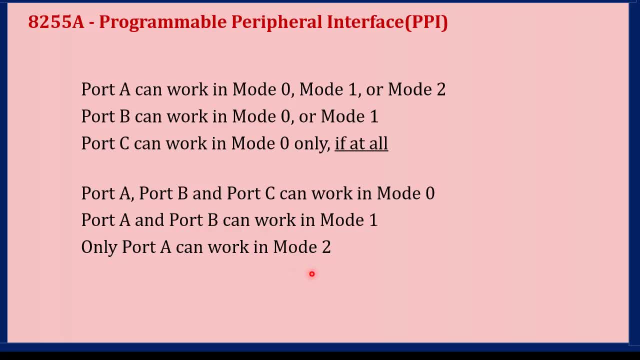 In mode 1, port A, port B are used. In mode 2, only port A is used for transmitting the data in and out. Let us see the architecture of 8255A: Port A, port B, port C. 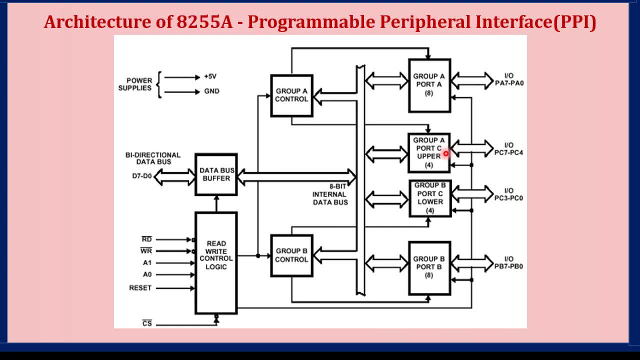 Each port consists of eight lines, Three ports, 3 into 8, 24 I-O lines. Again, these 24 lines are divided into two groups: Group A, group B. Okay, so here. group A- control block. group B- control block. 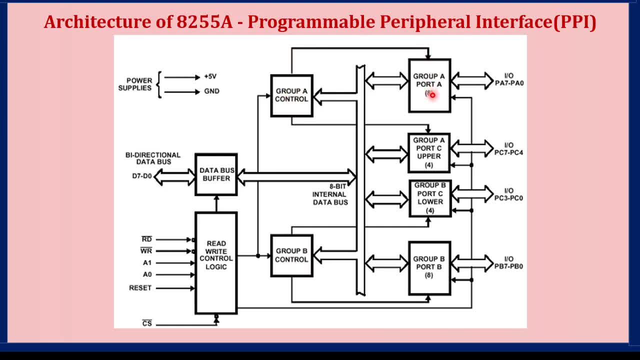 See group A. control is connected to the port A and port C upper lines. Okay, see port A: 0 to port A 7, port C: 4 to port C 7.. These are the 8 plus 4, 12 lines. 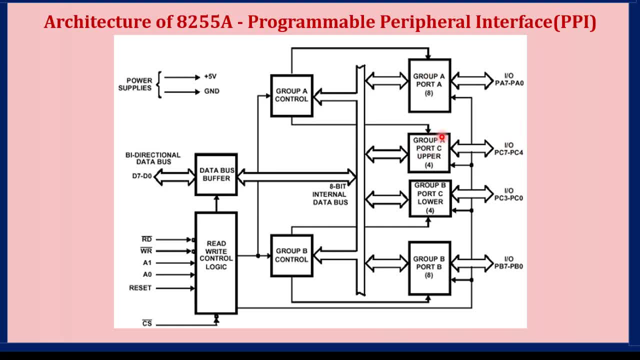 We can use this 8255 to transmit 12-bit data also. Okay, you can transmit 8-bit data, 12-bit data separately. Group A- control connected to the group A, which consists port A and port C upper lines. Okay, this is one group. 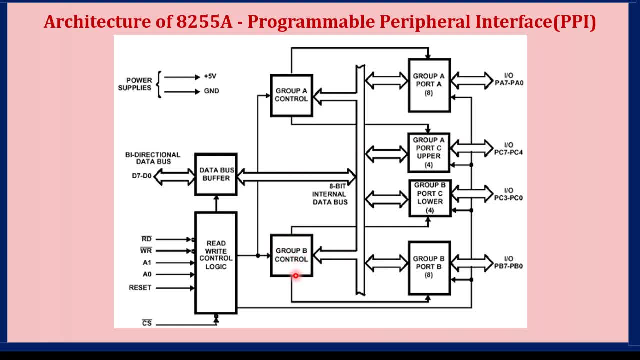 Next group B control Connected to port B and port C lower bits. Okay, that is PC 0 to PC 3. Port B having PB 0 to PB 7.. Right side lines are connected to I-O devices. Left side signals or pins connected to microprocessor. 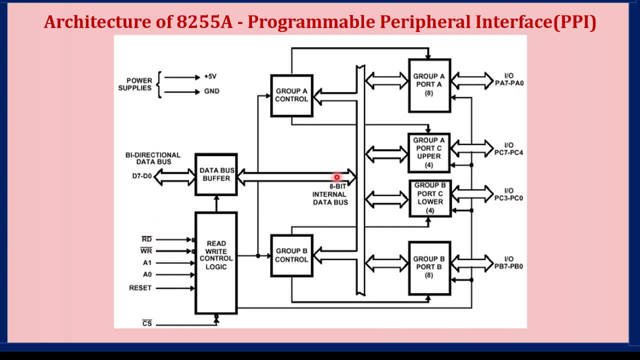 So 8255A exists between microprocessors And I-O devices. All of you concentrate on cursor. Okay, left side microprocessor is connected. So these pins or signals coming from the microprocessor, D0 to D7 lines of microprocessor connected to the 8255A through data bus buffer. 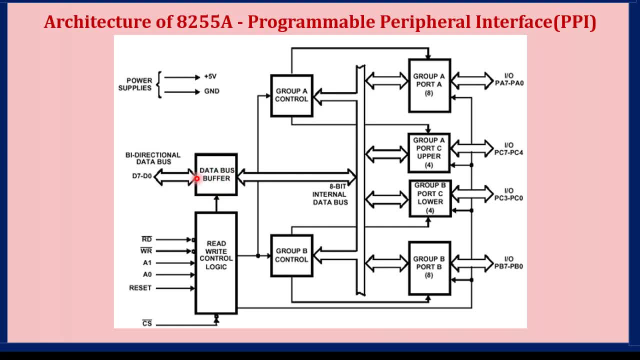 Bidirectional data bus buffer, which is used to transfer the data between processor and microprocessor, And 8255A Processor sends the initialization command words to the 8255A through this bus only, And also, whatever the data is to be transferred to the outside world using D0 to D7 lines. 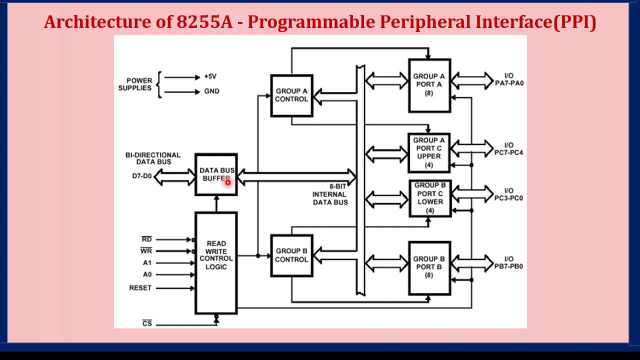 And receives the data through this buffer. Now read-write control logic. In case of receiving the data from outside world, Processor issues the read signal to 8255A through this signal. In case of sending the data to the outside world through this 8255A. 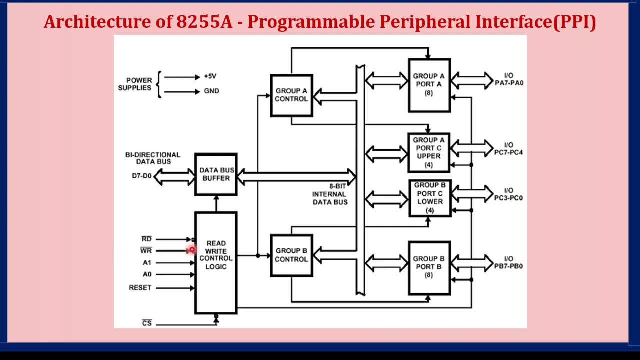 Processor sends write signal to this read-write control logic And A0, A1.. These pins are used to select 4TA, 4 to B, 4 to C And control word register. If these two bits are 00, 4TA is selected. 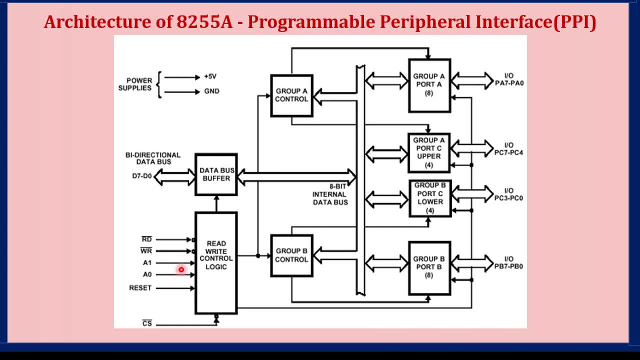 01,. 4 to B 10,. 4 to C 11, control word register of 8255A will be selected. To terminate the operation, processor sends this reset signal to the 8255A. So before going to start the operation of I-O transfers with 8255A. 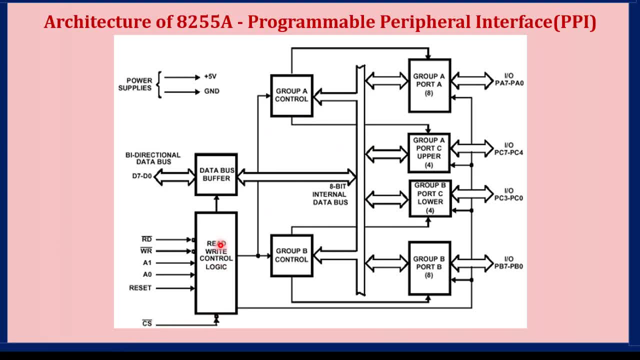 Processor sends the Chip select signal to the read-write control logic. to the 8255A through read-write control logic. Okay, So this diagram is very important. Whichever external device you want to interface, you have to use this interfacing device. 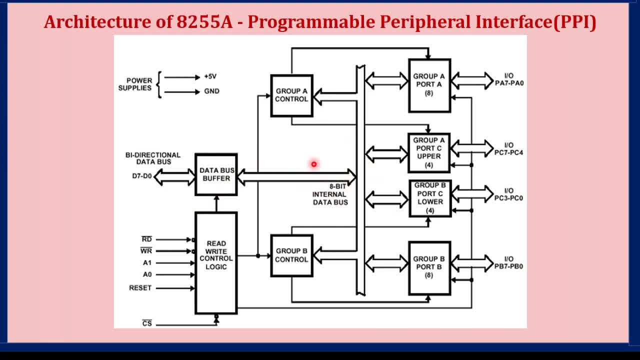 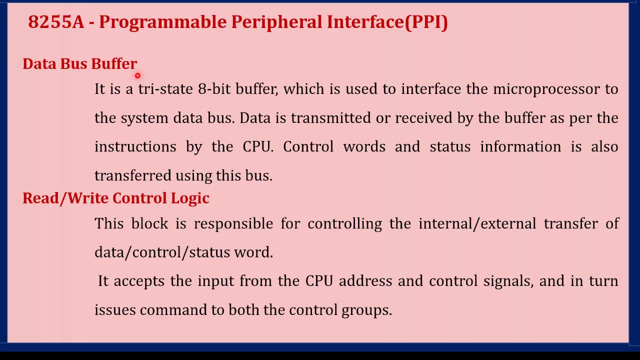 So there are chances to ask more examples. If you want to write interfacing programs in the lab, you have to learn this topic. Okay, Don't neglect this topic. Very, very important topic. I have written all the functions of blocks of 8255A. 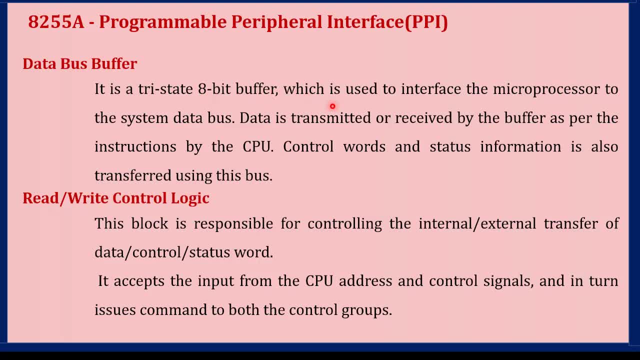 So data bus buffer, which is a tri-state buffer used to interface processor and read system. data bus Data can be transmitted or received by the buffer as per the instructions given by the CPU. So control words or status information of 8255A also be transferred. 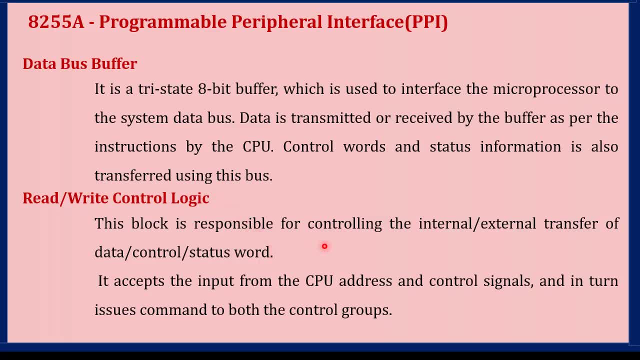 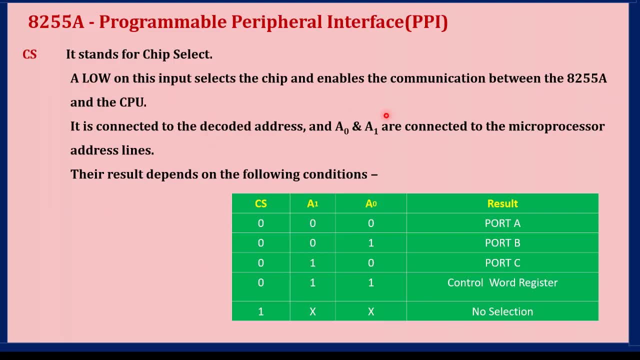 Through this bus Read-write logic responsible for controlling the internal external transfer operations, Chip select signal, which is always active low signal. It is connected to the decoded address. A0 and A1 are connected to the processor address lines. Okay, See, I told you A0, A1.. 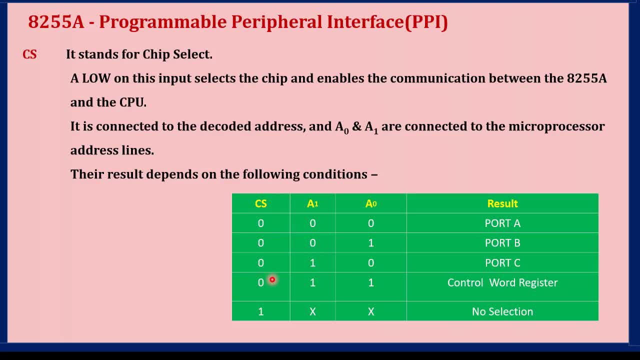 Chip selection signal: always low. Active low signal. There is a bar for this: A0, A1.. If both are 0, 0.. OTA is active: A0, A1.. Chip selected: 0, 1.. 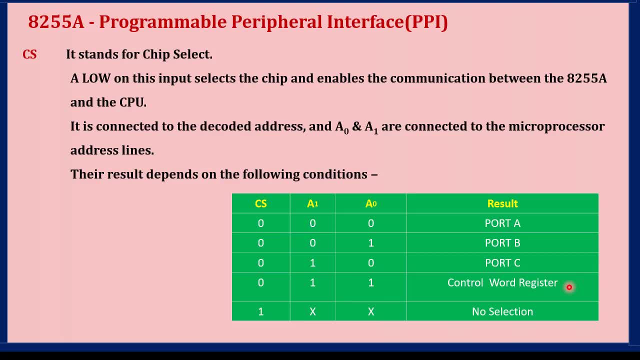 Port B selected 1, 0.. Port C selected 1, 1.. Control word register selected. Before going to use this 8255A processor needs to send the control word to the control word register of 8255.. 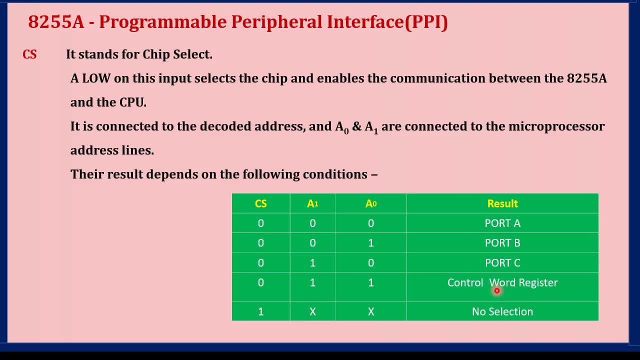 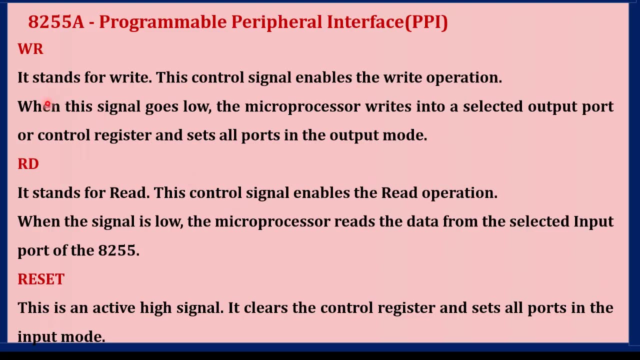 Okay, Then 8255 will act according to the control word or bits of control word register. This is called control word, Command word. Okay, So this is about read-write reset signals. I told you write signal Before going to perform write operation. microprocessor issues the write signal, which is a active low. 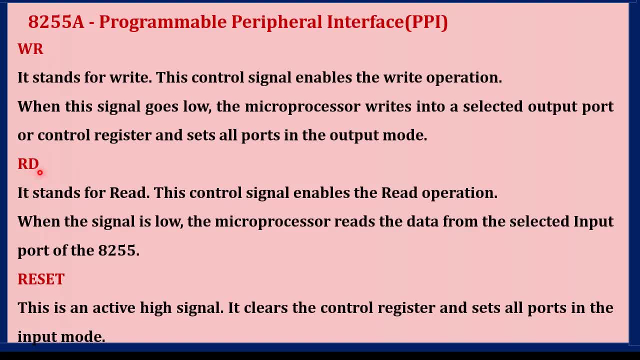 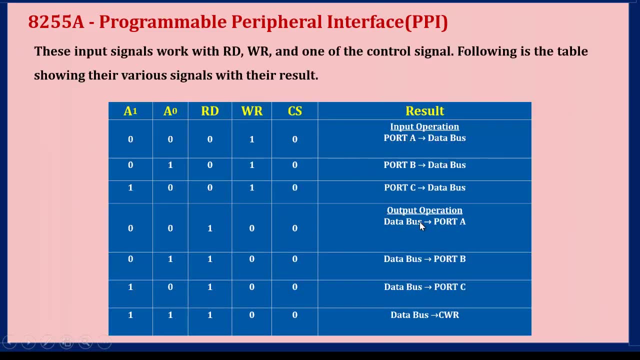 signal Before going to perform read operation. processor issues. read operation to the 8255A reset. This is active high signal used to reset all the activities of 8255A 5, 5 a. this table shows read operation and write operation based on control. 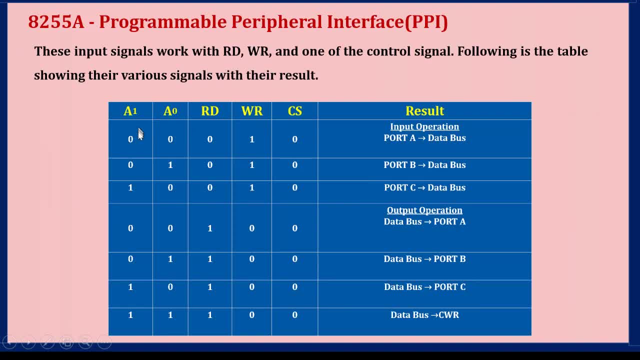 signal: read and write signals issued by the microprocessor. so a 0 a, 1 0 0 0, 1 1 0. then 40 a, port B, port C are selected. when read signal is 0, it performs read operation. read operation means the processor collects the data from the. 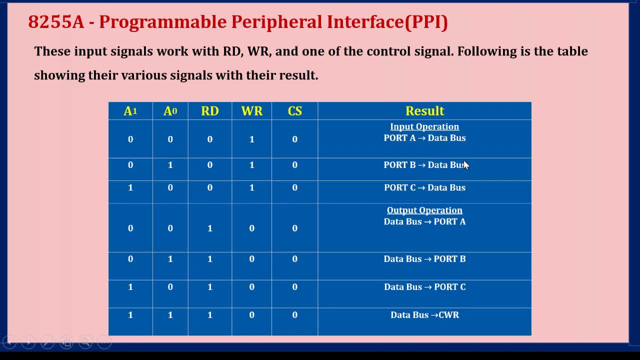 selected ports through its data bus. ok, next, coming to the write operation. in case of write operation, write is a active low signals. that's what these are, all zeros. at the time, our read bar is 1, 1, 1. ok, now 0, 0, 40. a selected: 0, 1 port B: 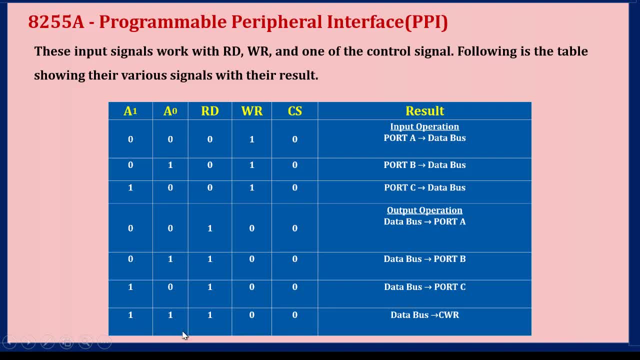 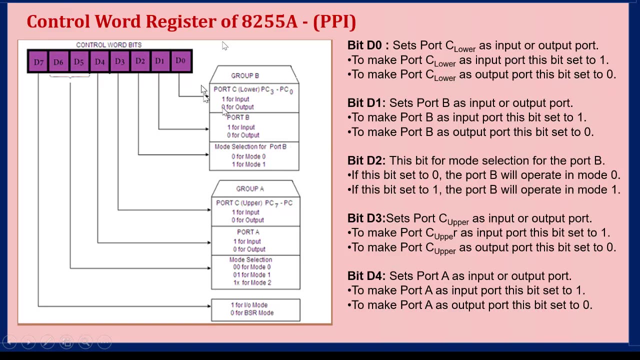 selected 1: 0. port C. selected a: 0, a, 1, 1, 1. then control word register is selected, so to write: the data process sends the data to the selected ports through its a data bus buffer. ok, next. so this is the control word register of 8255, a very, very important group to lead up a practice. 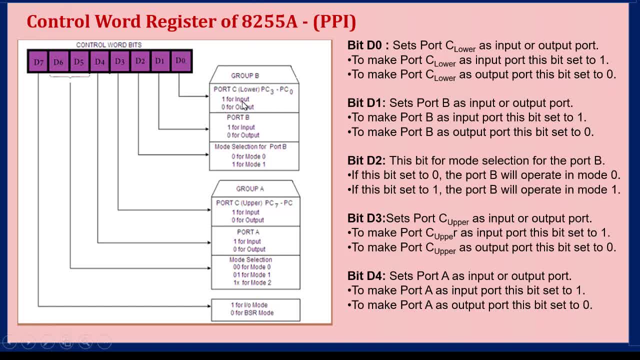 in the ok. so D 0 bit indicates for: to see lower bits: PC 0 to PC 3 L. actually, if this bit is one, this four lines acts as a input lines. this bit is 0, 0, 0. this four lines actuallyالthe output lines means input lines, means those. 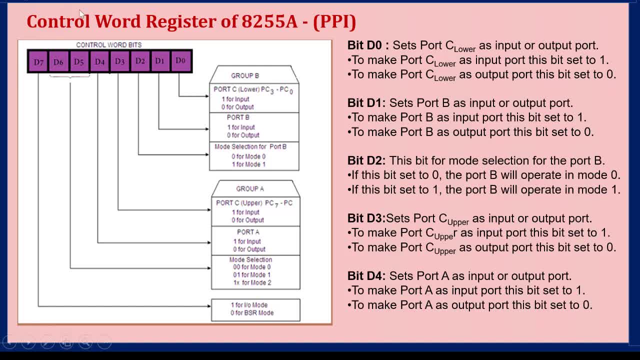 lines are used to receive the data. output lines means those lines are used to transmit our data. next, D: 1 bit, the port B. if this bit is one, port B is used as input port. if this bit is 0, port B a is used as output port. okay, so i told you P. if this bit is one, then thisnant theinos is 1. both B is used as input port, which, if this bit. 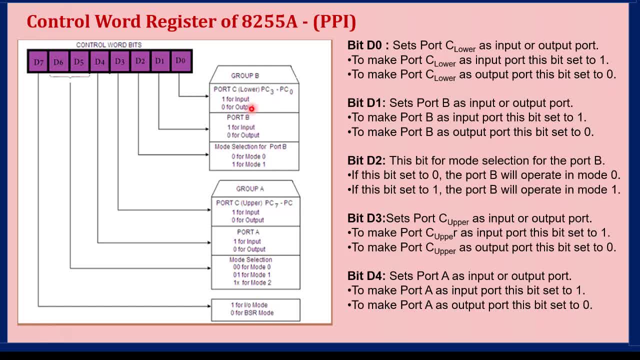 told you, these two lines are grouped together, called as group B signals. next, d2 bit is used as mode selection for port B. if this bit is 0, mode 0 will be selected. if this bit is 1, mode 1 will be selected. we already discussed about mode. 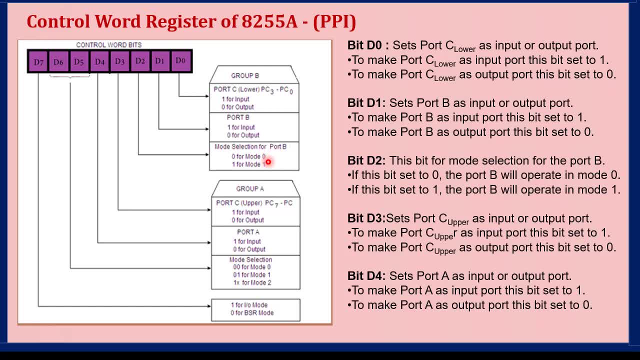 0 and mode 1. again refer those modes. ok for port B. ok now. d3 bit is used for selecting. ok, PC 4 to PC 7. upper lines of port C are used as IO lines. if this bit is 1, d3 bit is 1. these four lines are used as input lines. d3 bit is 0. these: 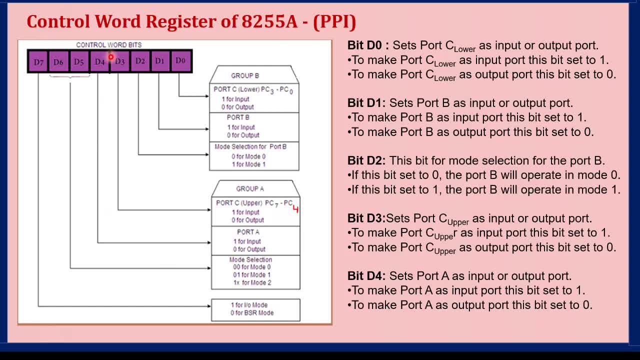 lines are used as output lines. coming to the d4 bit is used for Port A. These bit determines Port a is used as input port or output port. ok, input port and accomplishment data and research s card on the output port and a data and sentry donkey ok. 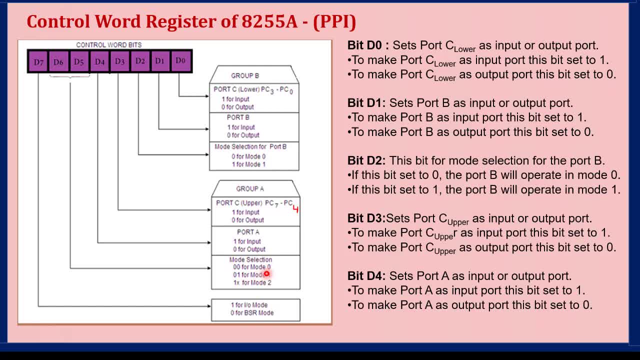 D5, D6 bits. are you dette first selecting though modes: mode 0, mode 1, mode you. if these two bits are 0, 0 more 0 selected 0, 1 more one selected one cross syndicate, Oh des you Across may be 0 or 1.. If 10 or 11 or mode 2 will be selected. So again, refer about all these modes, In all modes, how the ports are operated. 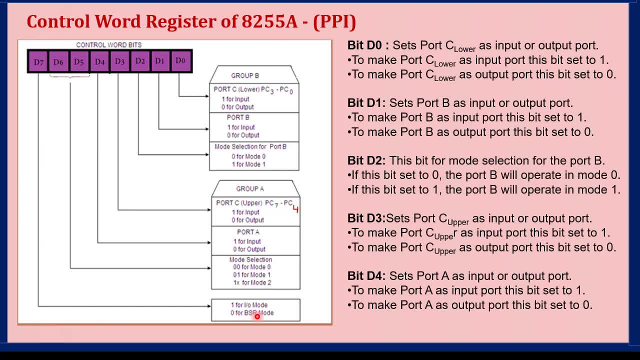 Okay, so D7 bit is used to set IO mode or BSR mode. Basically, 8255A operates in 2 modes: IO mode and BSR mode. In IO mode again, processor enters into 3 modes: Mode 0, mode 1, mode 2.. 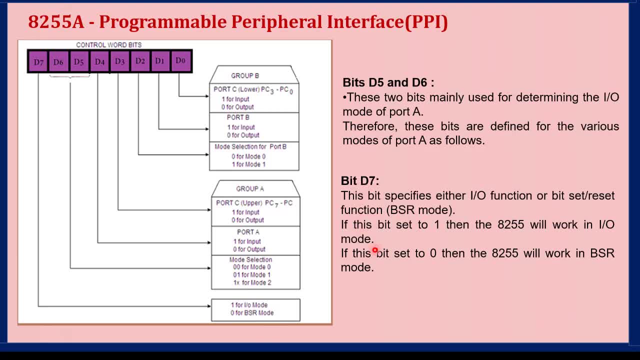 In BSR mode, see here- D7 bit is set to 1.. 8255A operates in IO mode. IO mode means again, it is divided. It is divided into 3 modes: Mode 0, mode 1, mode 2.. Okay means, in IO mode we can select any kind of mode 0, mode 1, mode 2.. Okay, if this bit is reset, that means 0.. 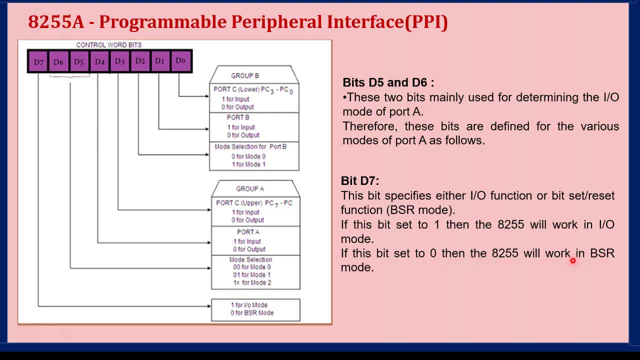 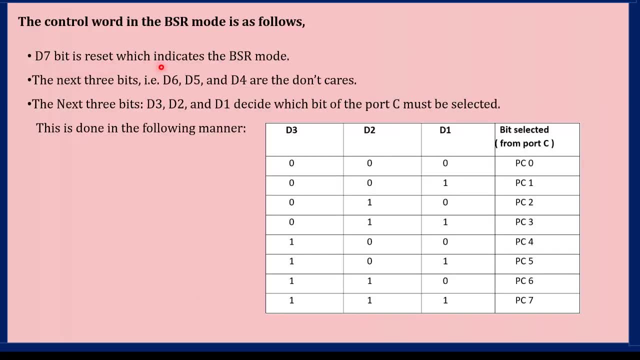 Then 8255A enters into BSR mode. Means bit set reset mode. Okay, in this case, D7 bit is reset means 0.. Then 8255A enters into BSR mode. In case of BSR mode, D4,D5,D6 are tuned case. They are not at all used. Okay, next 3 bits of a farewell: D2,D3. 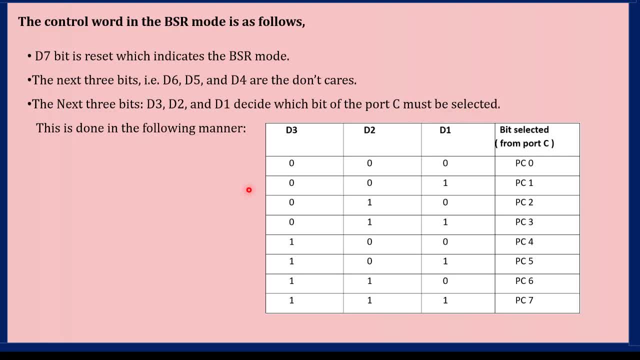 Decide which bit of the port C must be selectedOkay, if you want to select any one of the port C, then contain the RGB". Then you need to limit the D7 bit which is still live, Then set off the D7 bit. 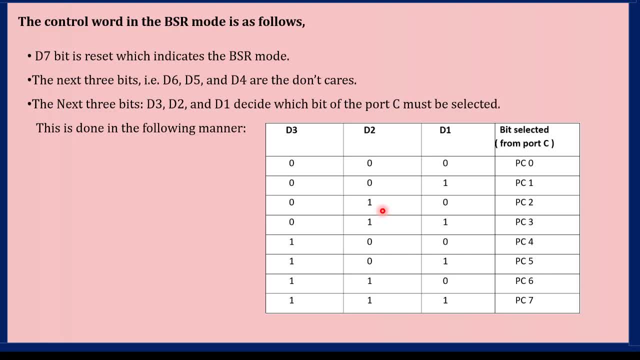 If you want to use any bit- D1 is also in decided mode- than enter Pokemon mode and 5 remains to accessible mode. Then set off D7 bit, which is 8255A. Press M1.. Press M2.. d6 bits of the control word registers are not used. okay, so d1, d2, d3. so if these three bits are zeros, 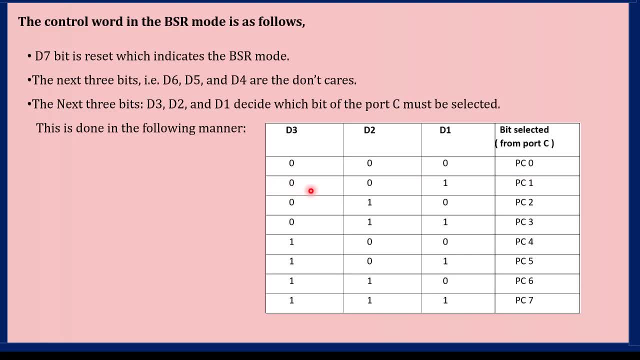 pc naught line will be selected. 001 pc1 can be used to transmit one bit. okay. next, 010 pc2 will be used, okay. likewise, for all these combinations, we can use any one of the 4 to c line. okay. so remaining d0 bit together, what them 8 bits? d0 to d7, so you could a d4, d5, d6, don't guess. d1, d2, d3. 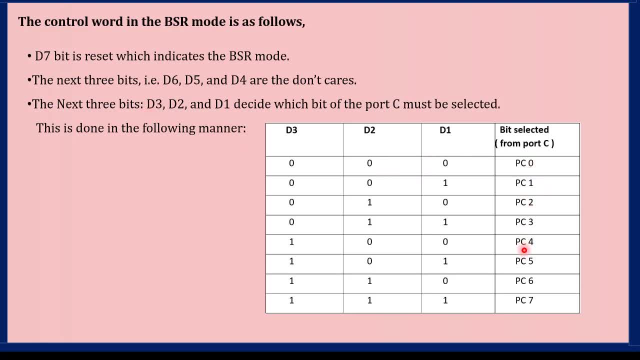 are used for selecting lines of 4 port c. okay, d0 bit together: set or reset. d0 bit can be set to one or reset to zero. okay, based on that, any one of the 8 bits of port c can be set or reset depending upon the d0 bit. so port c line can be set or reset. 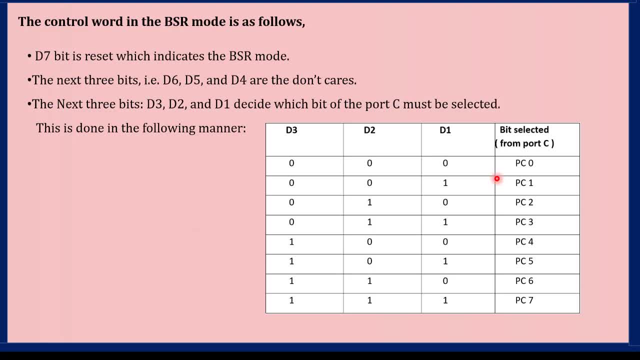 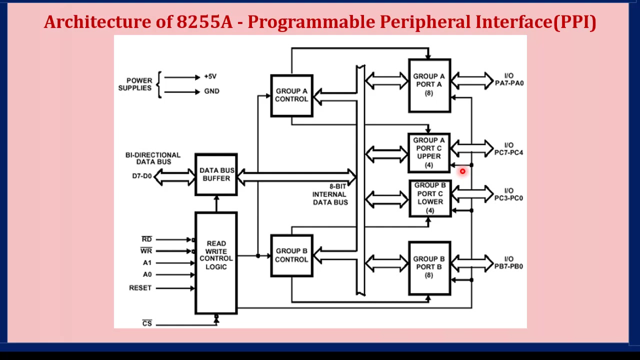 depending upon the d0 bit. d0 bit. one night a it'll climb. select, uh, set just them. d0 bit zero: a particular line reset out. this is how. 8255 a is a programmable peripheral interfacing device. programmable can be programmed by a processor. that means processor sends the initialization command words.